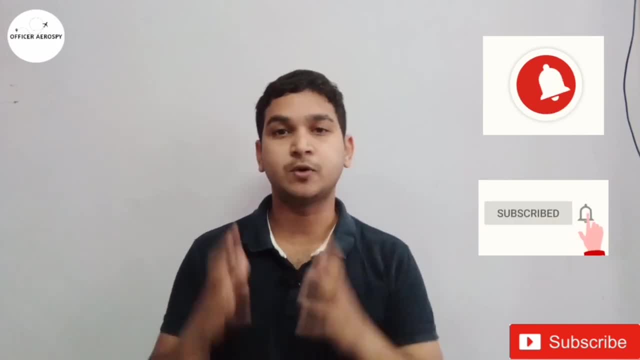 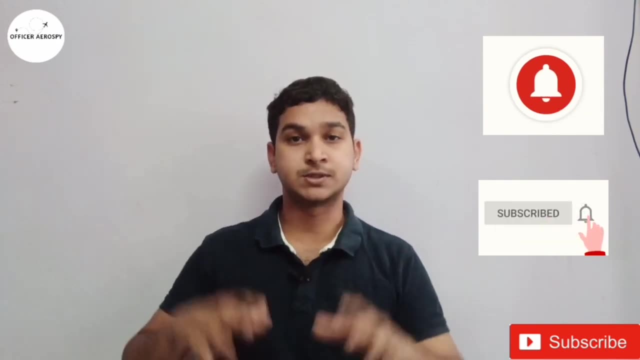 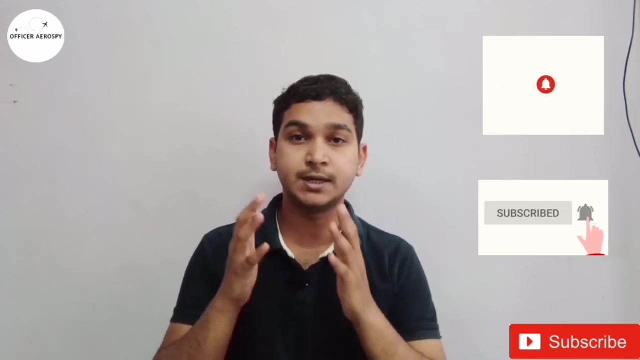 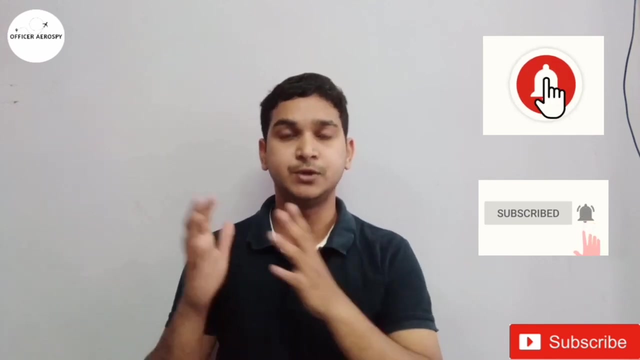 So before that, I would like to tell you to subscribe to officer aerospace channel, like share and comment in the section below how you feel the videos, because these videos are all related to the aerospace engineering branch and everything I will cover in depth and in very detailed conceptual way. So this is for you guys who are new to this channel, Please. 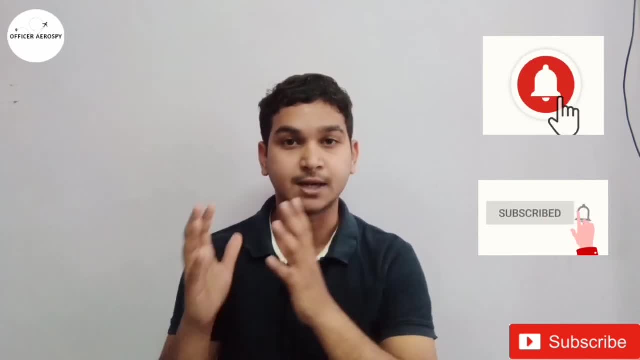 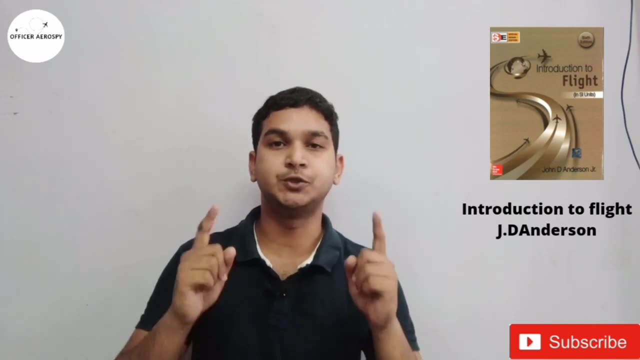 subscribe to officer aerospace channel like, share and comment In the section below. So let's begin with the books. So book number one, introduction to flight, by John D Anderson. Of course this book is called a Bible of all aeronautics branch because this book includes all the ample of knowledge and all 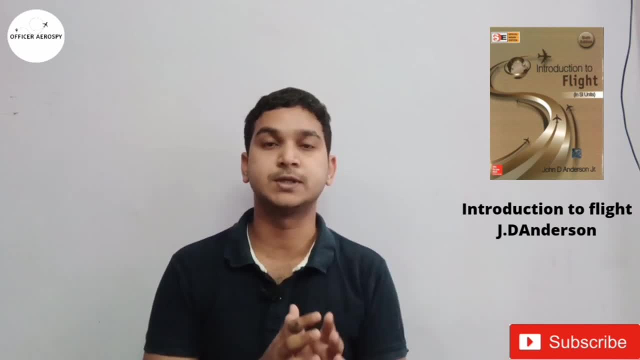 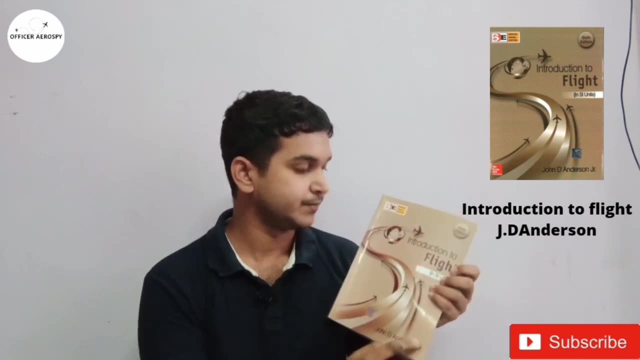 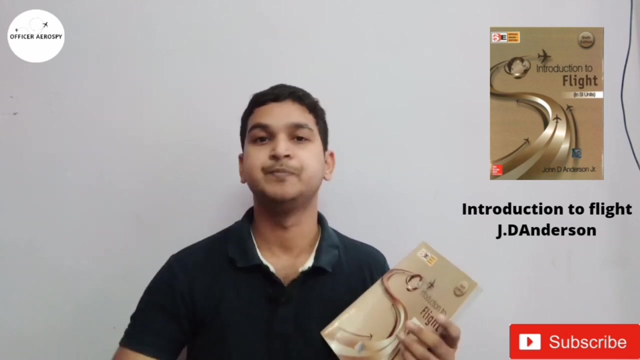 the field, the whole overview of aeronautics field. So this book looks like this: The introduction to flight by John D Anderson, And this book covers each and everything: basic level understanding of aero field. So it starts with a stranded. 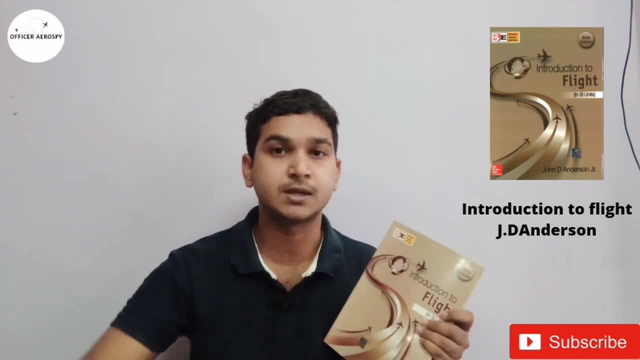 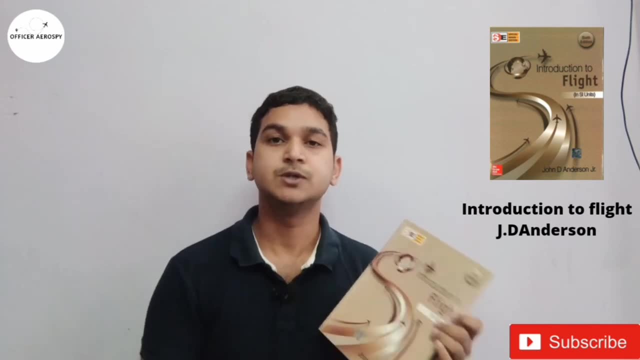 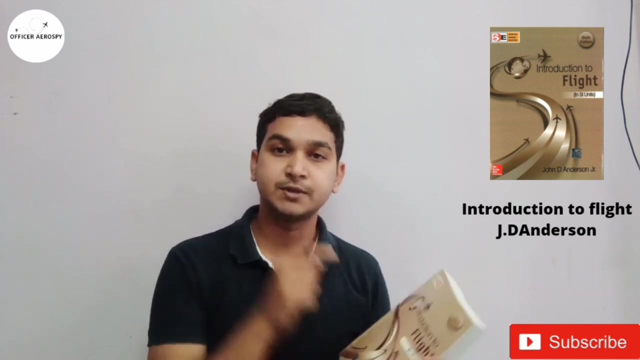 atmosphere and goes on up to hypersonic vehicles, performance and structures. Everything is covered in introduction to flight by JD Anderson. So if you are starting with a scratch in this first semester or you know engineering syllabus as per concern, so start with this book. you will get a basic knowledge of what is called aeronautics. 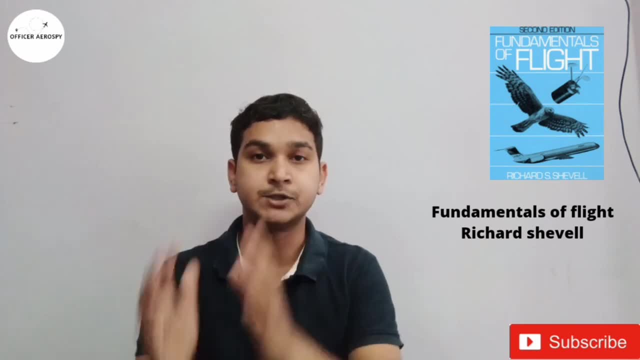 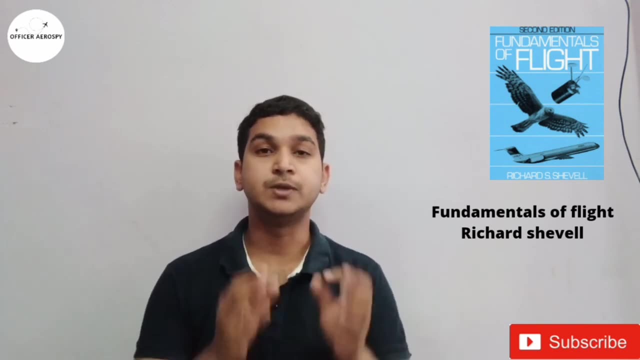 So book number two is fundamentals of flight by Richard Shavell. So Richard Shavell has written this beautiful book with a minimum number of equations, So it is very helpful to understand the concepts related to the aero field, whether it may be a drag, whether it may be a lift. 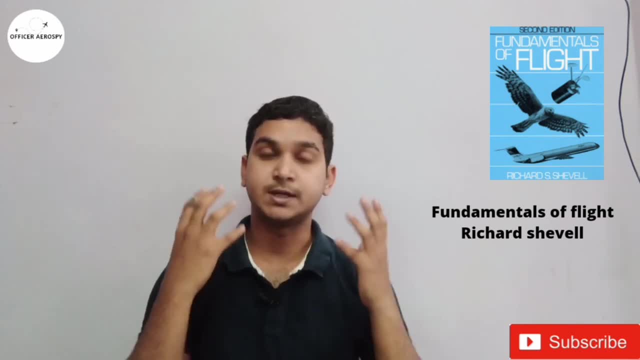 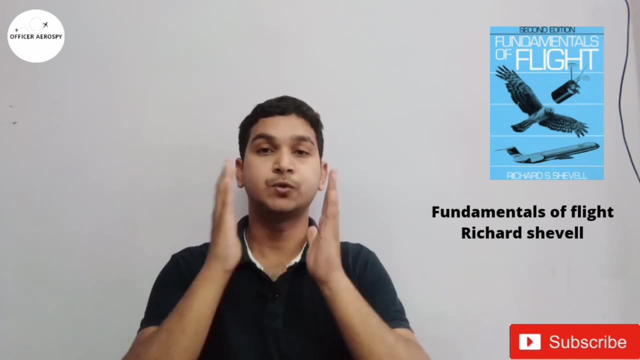 whether it may be a performance of an aircraft, whether it may be a structure of an aircraft and the rocket trajectories and orbits, whatever it is. But this book helps you to understand the insightfulness of all the concepts. So this is how the book looks like. 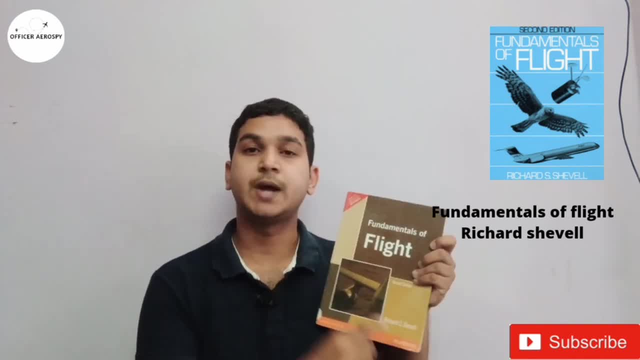 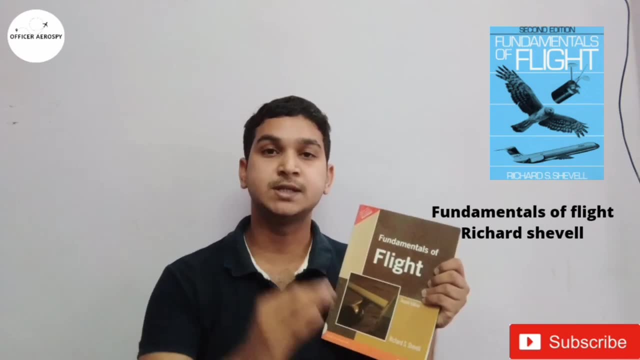 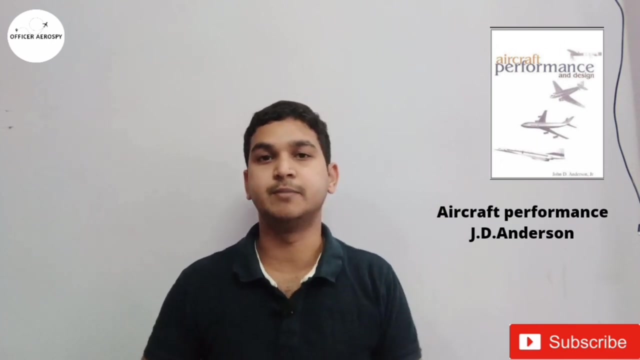 fundamentals of flight by Richard Shavell. So I would recommend this. book is very, very helpful for each and every student to understand the basic knowledge of aero field. So book number three is aircraft performance and design by John D Anderson. So somewhere you'll get this book around. what the cheaper prices? but I would like to 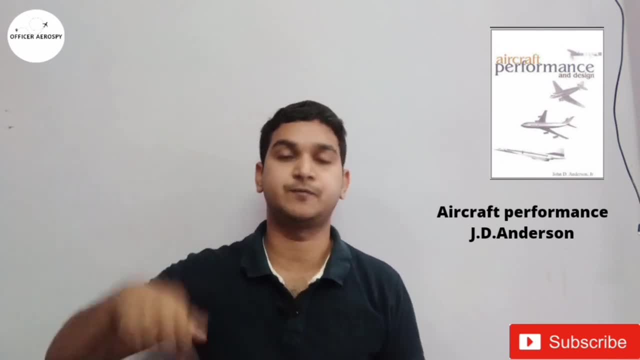 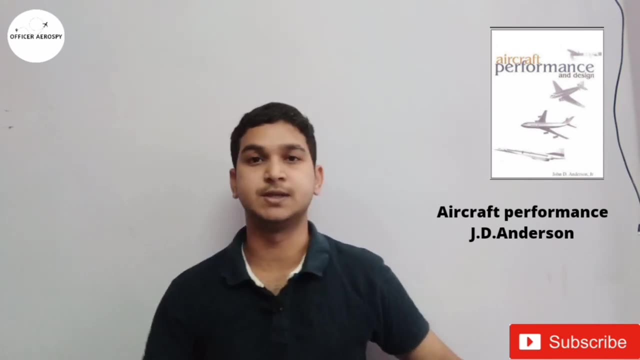 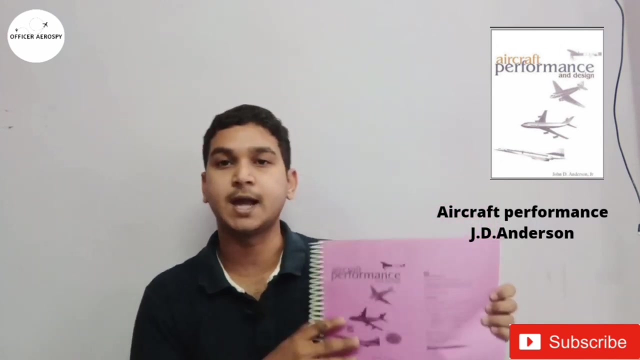 to recommend you to take this book in the pdf format given in the description below, so the cost will be minimum for your learning. so in my btech studies i took this book in a xeroxed copy. the book is called aircraft performance and design by john d anderson. so this is the book and this book. 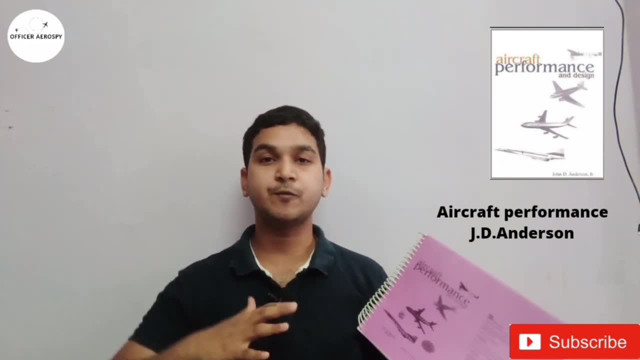 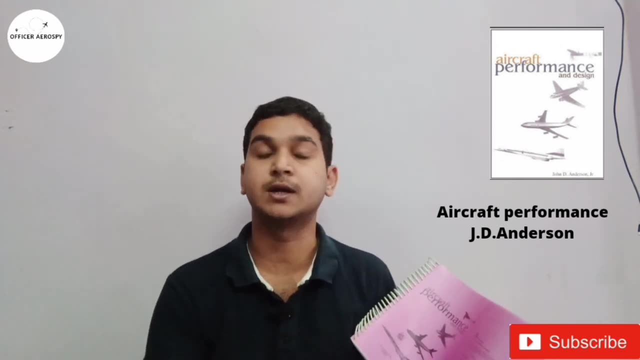 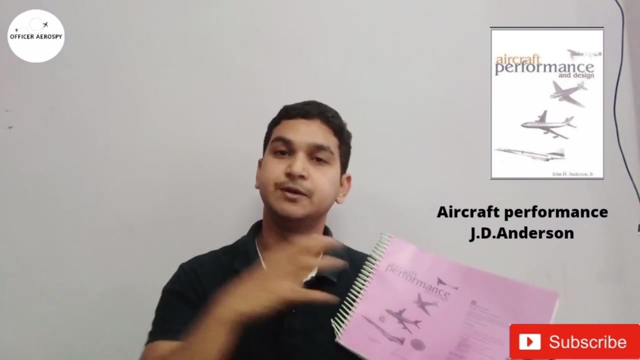 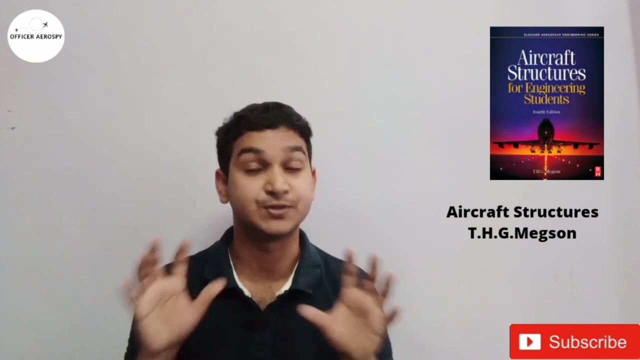 is all about the performance of the aircraft. so aircraft when it is going in a different atmosphere, how the performance takes place and how this affects the other parameters of the aircraft. so i would recommend this book is also very, very important to understand how aircraft performs in different field. book number four is very important. the name itself indicates it is very important. 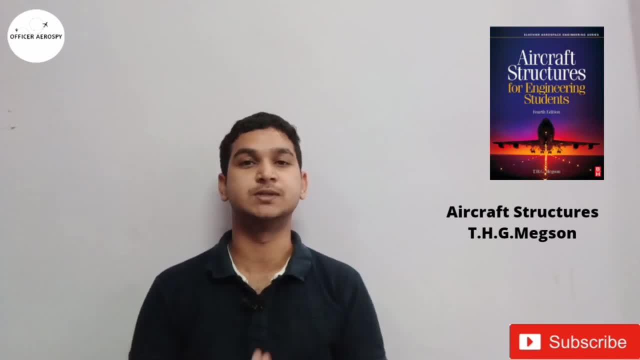 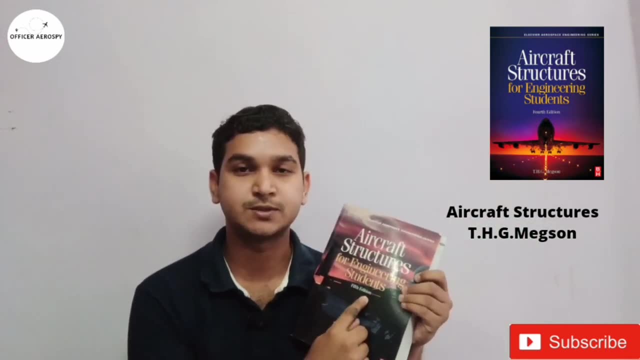 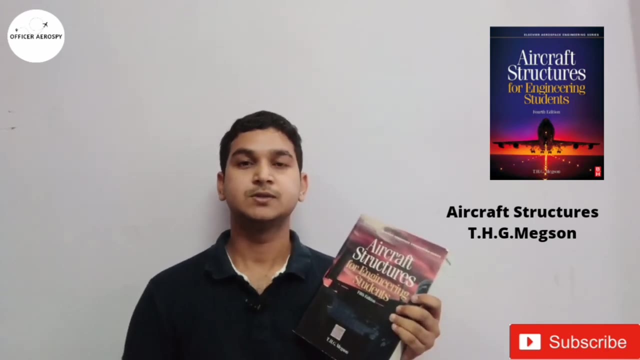 the name is aircraft structures for engineering students by th g maxim. so this is the book called aircraft structure for engineering students by THG Maxson. So many students feel this book is very, very toughest part in the aero field. So don't worry, we'll make it simple in this officer aero spy lecture series. 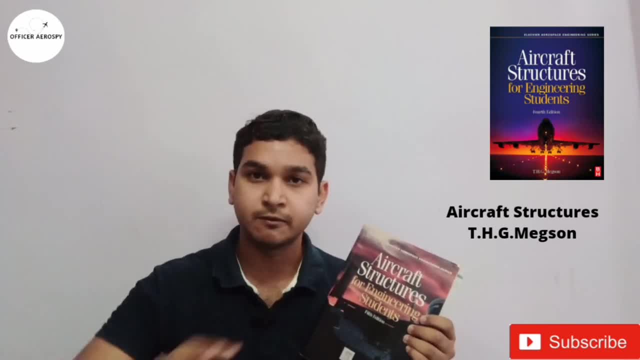 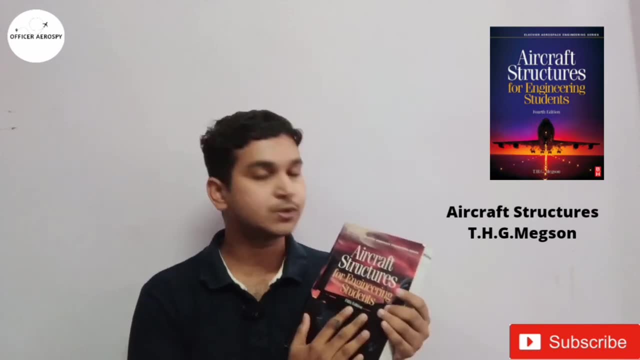 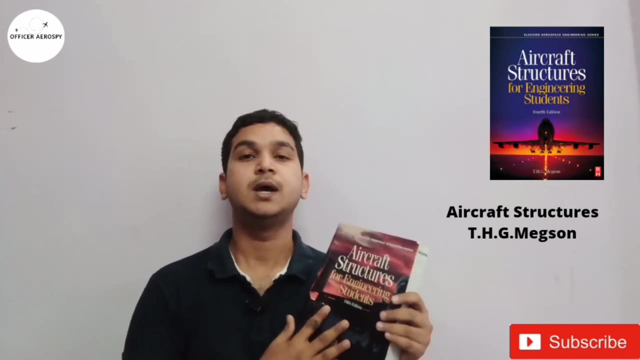 of on the aircraft structures. I will cover from the scratch to the finish level, how to solve the problems, how to structure the aircraft. So in this book it is very clearly written what the materials we have to use, what are the loads imposed on the aircraft structures and how to. 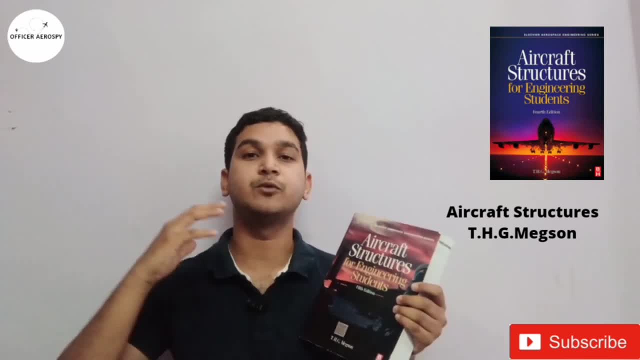 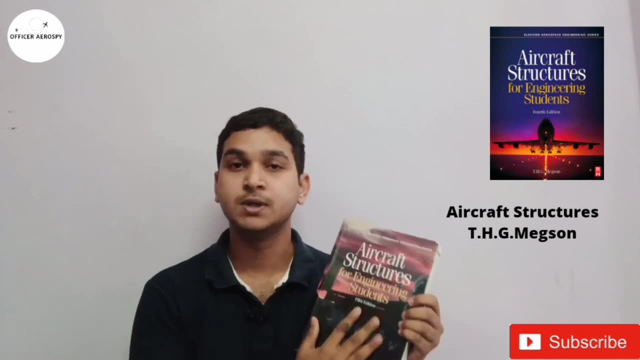 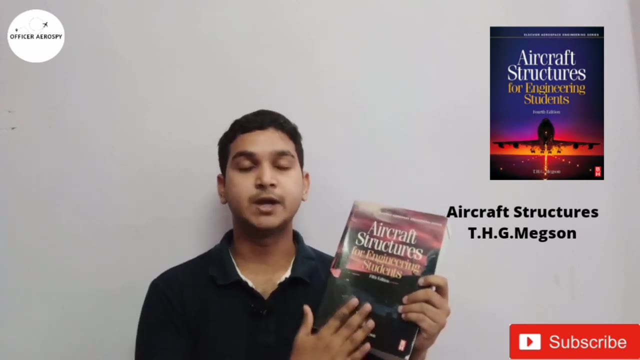 design a fuselage, what are the problems arises and how to analyze the problems when you design a wing structures. So all, each and everything it is given in this book. So this book I would recommend to every students studying aeronautical engineering or aerospace engineering. This is very good book. 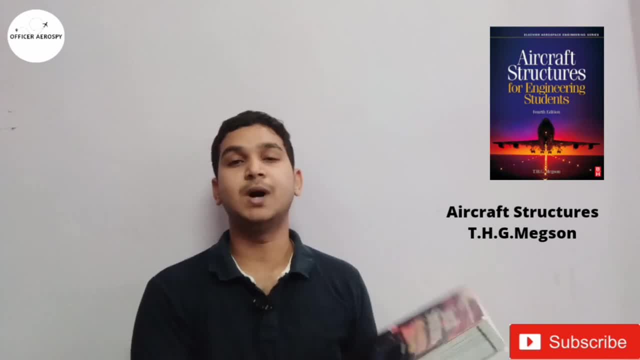 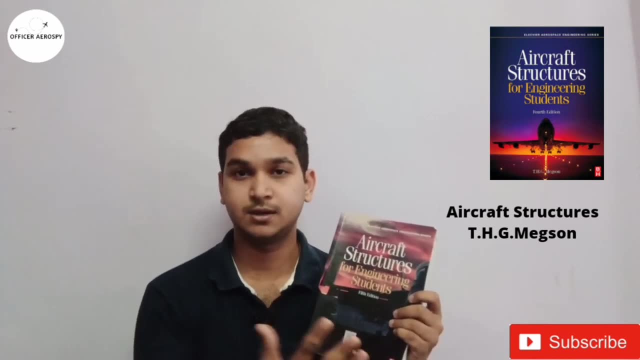 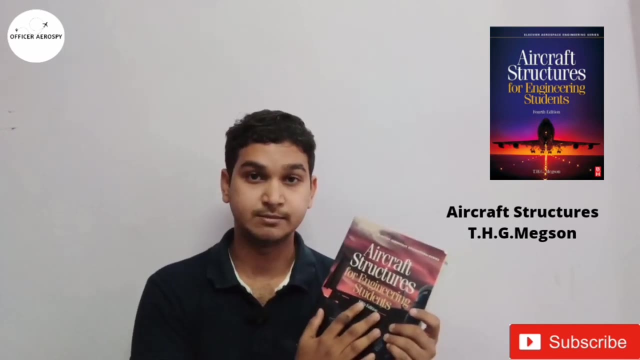 and you have to finish it to the mark. So one disadvantage of this book is this book is very costly in the India and outside, I would say, and when you search in Flipkart and Amazon you will get this book for around 11,000 rupees sometimes. So don't worry, I have given the link in the 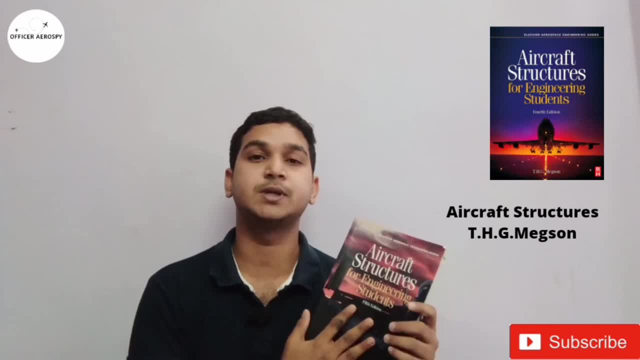 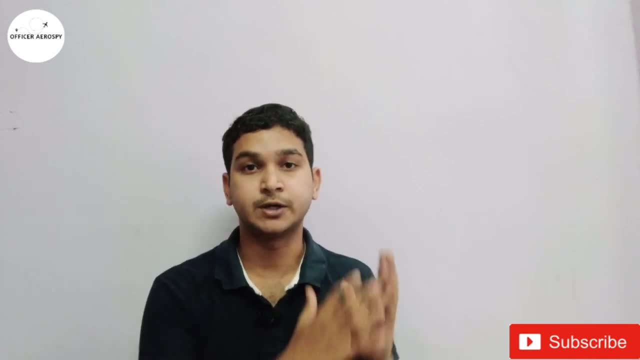 description below. Please go to the description and you will get this book for free. So don't worry guys. these all books and all the concepts related to aero are covered in the lecture series coming soon on basic aeronautical engineering, Aerodynamics, basic structures and performance. every subject I will cover in a very detailed 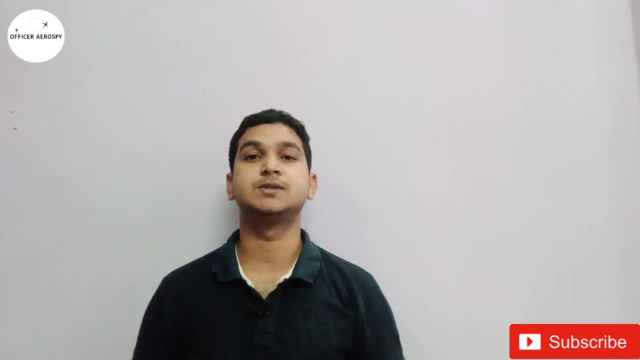 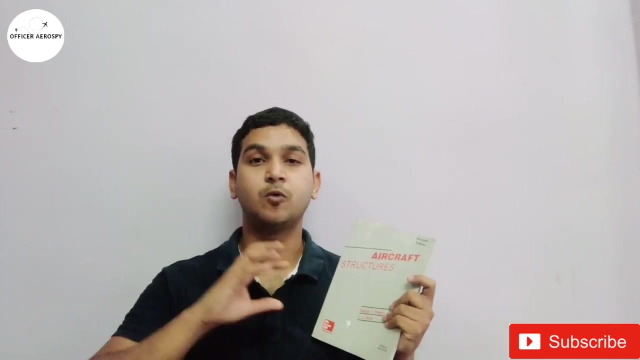 manner. So next book number five is the aircraft structures by David Perry. So this is the book called aircraft structures by David Perry. and what is the main difference between the TGH Maxon and Perry book is the one thing: the Perry covers the whole problems involved in aircraft. 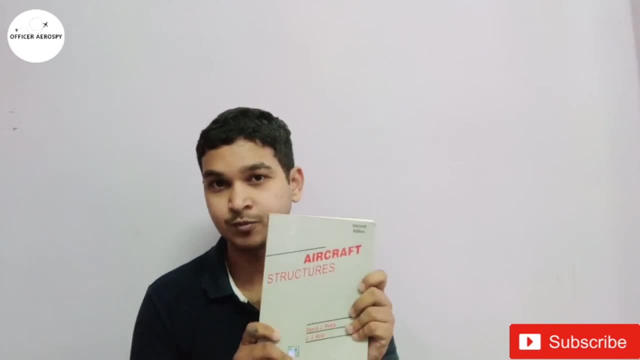 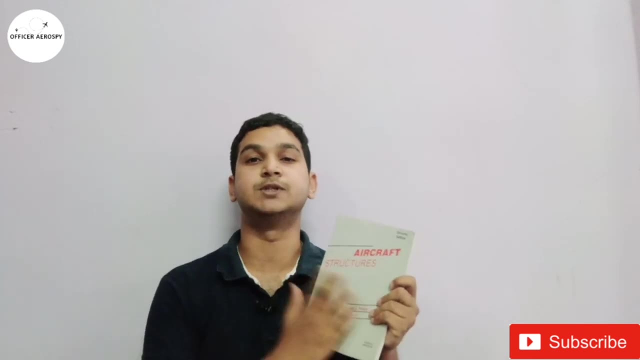 structures. So this book, if you are going to understand this book, this book comes with n number of problems and if you are fond of solving n number of problems, you are in a right track and go for this book. So book number six is mechanics of materials. 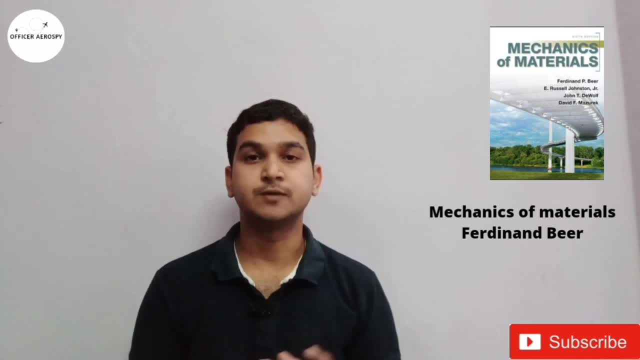 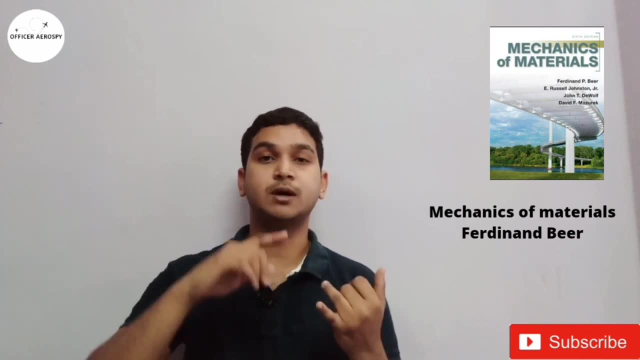 So first, if you want to understand the aircraft structures from the basic, you have to learn the mechanics of materials. So in mechanics of materials it will come with a concept of torsion, it will come with a stress strain, it will come with a bending. 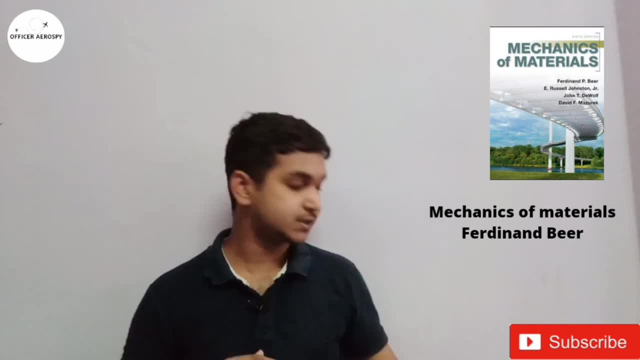 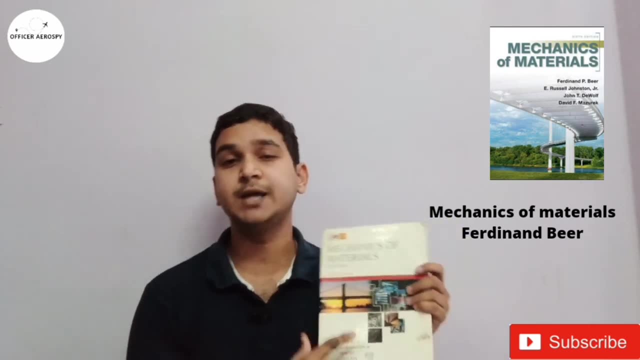 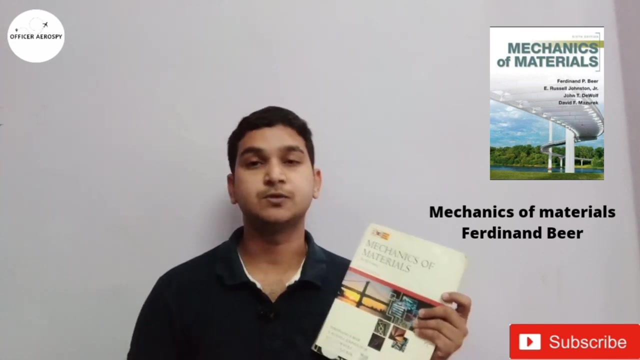 it will come with a column energy methods, each and everything. it is covered in this book called mechanics of materials from Fred Rando Beer. So I use this book to understand the basic knowledge of stress, strain, torsion, column energy methods, everything. So I would recommend 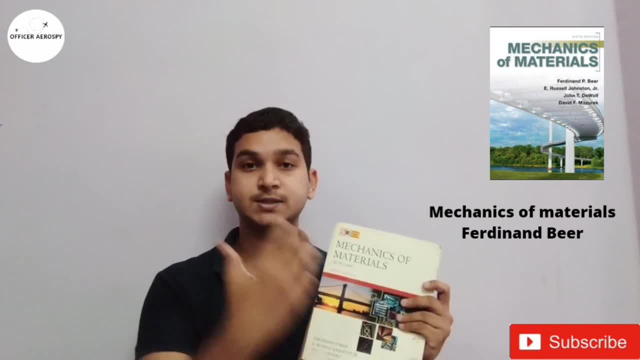 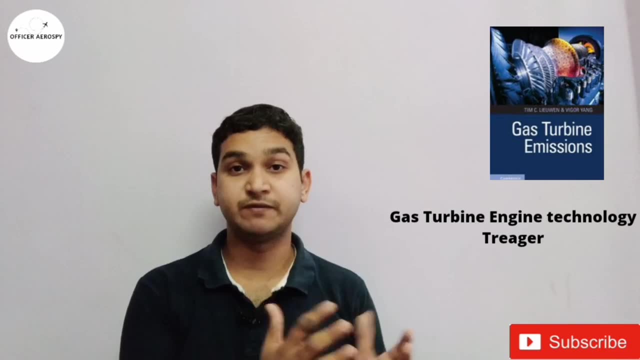 this book to all the aero students who want to understand the aircraft structures in deep. So first you have to understand this mechanics of materials. Book number seven is aircraft gas turbine engine technology by McGraw-Hill publications. So this is also very good book. 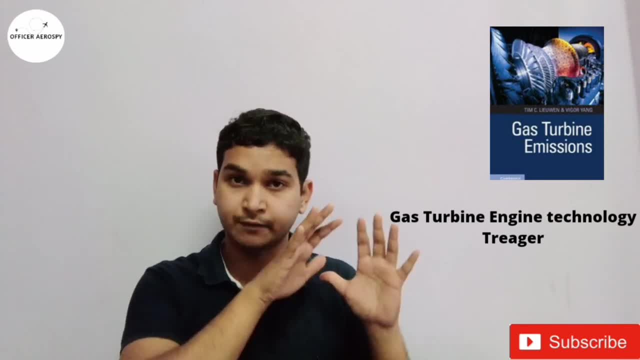 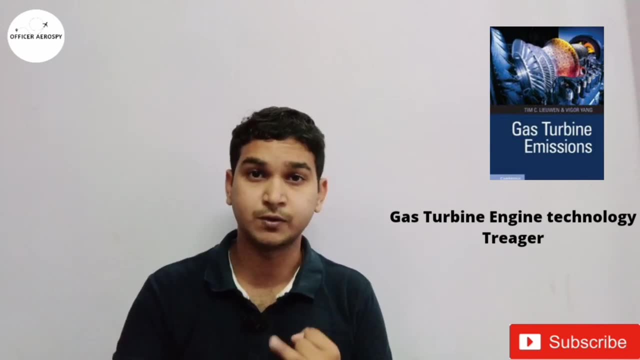 So if you want to study this book in very deep manner, first you have to understand the thermodynamics, how it works. So you have to understand how the basic engine works, on which principle it works, everything. So if you are in the notion that you don't understand the concepts, go through my videos which are on jet engines and understand from the basic level why I am talking about this concept. So if you are in the notion that you don't understand the concepts, go through my videos which are on jet engines and understand from the basic level. So if you are in the notion that you don't understand the concepts, go through my videos which are on jet engines and understand from the basic level why I am talking about this termsm.